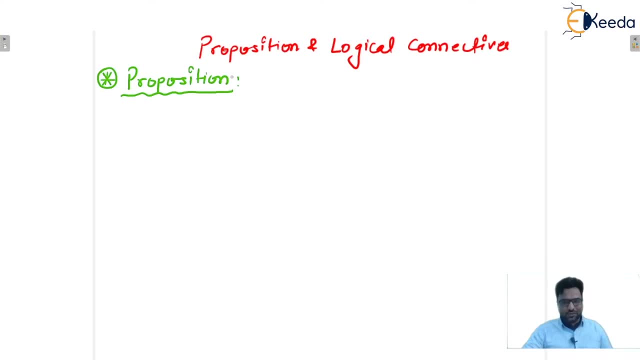 But not both. that is known as proposition. So what is the meaning of declarative sentence? A declarative sentence means a sentence that declares some fact, Isn't it Ok, so write down. Yes, a proposition is a. we can say that declarative sentence. that is either true or false. 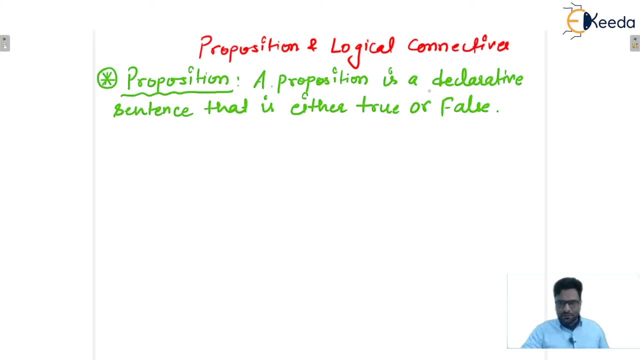 Isn't it? And the meaning of declarative sentence is what We can say: that declarative sentence means, yes, a sentence that declares some fact. So we can say that a sentence that declares some fact, Isn't it? So that is proposition. 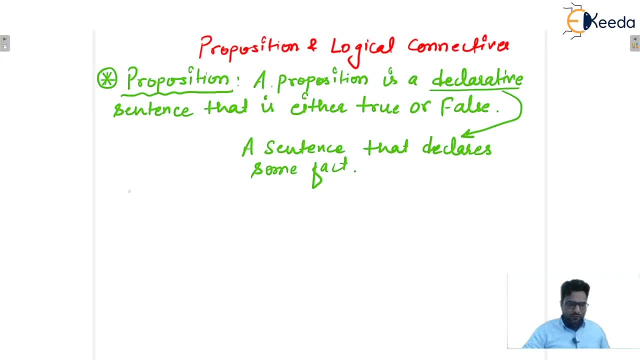 So let us take some examples of proposition. First one we can Write down. Let us consider example number one. You only tell me, Let's say, this statement is given to you- Washington is the capital of United States of America. So you know very well, this statement is true. 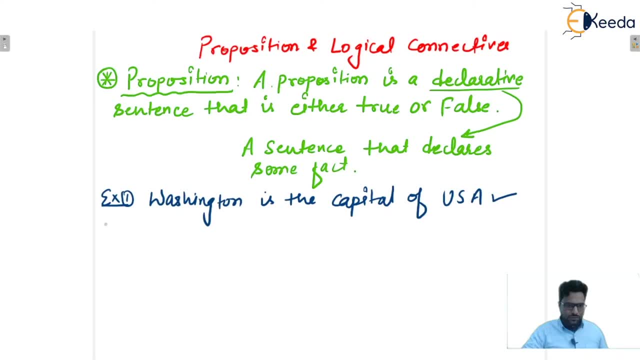 Yes, that's why we can say that this one is your proposition. So let us consider next example. Let's say example number two. So we can say that, let's say, one plus one is equals to three. so you know this statement. 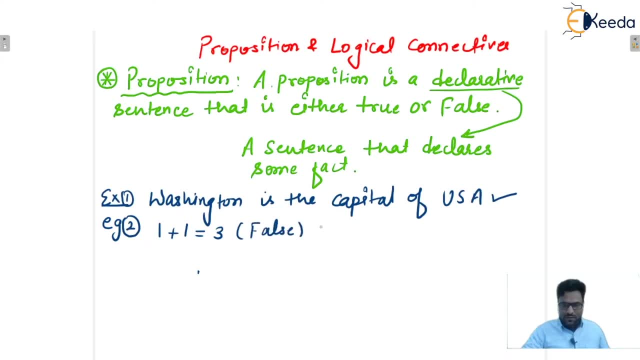 is what we can say? that false? and because of this one is false, So we can declare that this statement is a proposition. Next one, You can take. next example. You only tell me, let's say one plus three is equals to four. 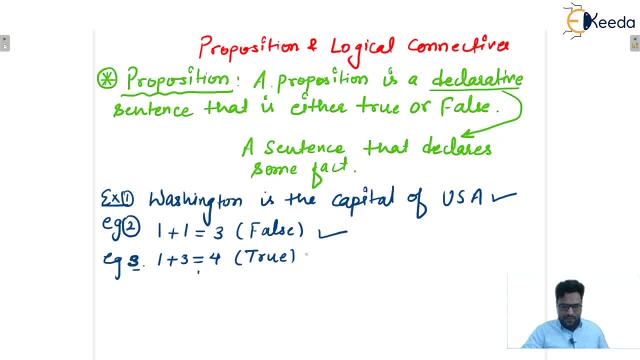 So we can say that, yes, this statement is true because of that, So we can call it proposition, Isn't it? Next one, Let us take one more example. You only tell me, Let's say, one statement is: what time is it? 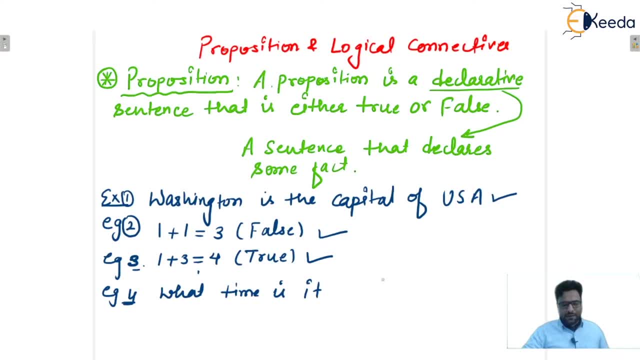 Isn't it? What time is it? That is the next statement. So you only tell me what time is it. It is, Yes, we can say that, not a proposition. Why? Because because we can say that these are. this statement is not a definition. 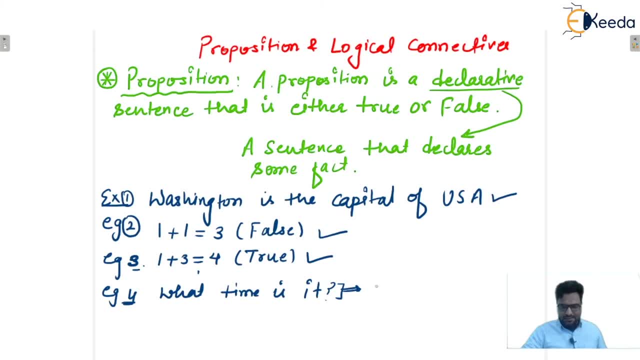 It is not a definition, It is not a declarative sentence- Yes or no- Because this statement does not declare any fact, Yes or no. So we can say that this one is not a yes declarative sentence, Isn't it? 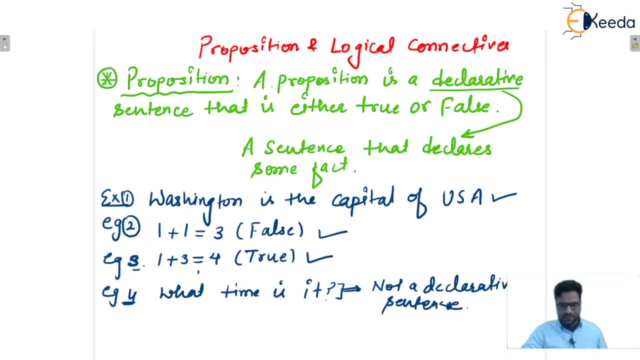 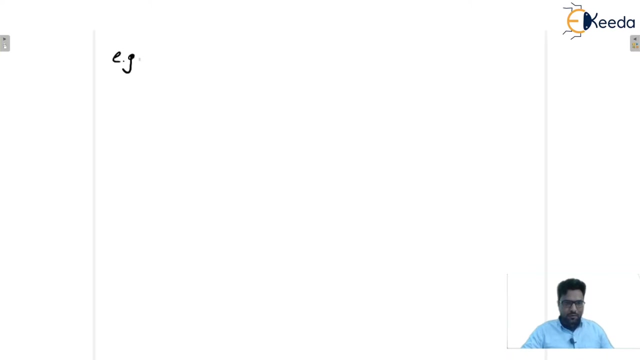 Declarative sentence. because of that, we can say that this statement is, yes, not a proposition, Isn't it Not a proposition? Yes, okay, okay. so let us move to the next statement. okay, so write down next one. yes, let us consider one more example. let's say next example, let us consider one more statement. 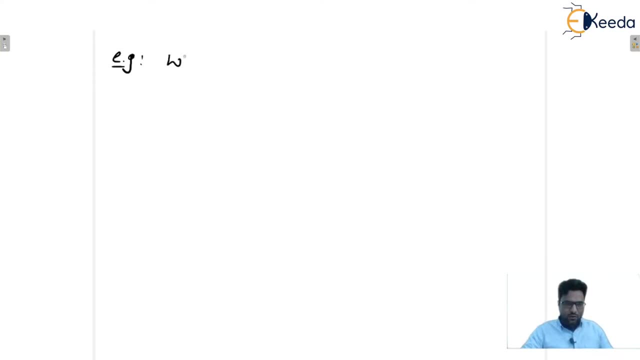 let's say any question. let's say: where are you going? where are you going so we can say that this is yes? this statement is neither true nor false. that's why it is not a proposition. next one, let us consider one more. let's say any example related to commands. go there, yes or no? 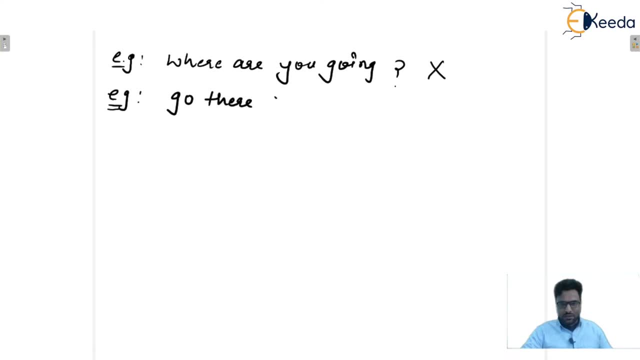 go there, isn't it? so we can say that this one is not a proposition, because this is neither true nor false. that's why we can say that this one is not a proposition. next one: let us consider one example related to commands: yes or no. go there, isn't it? so we can say that this one is not a. 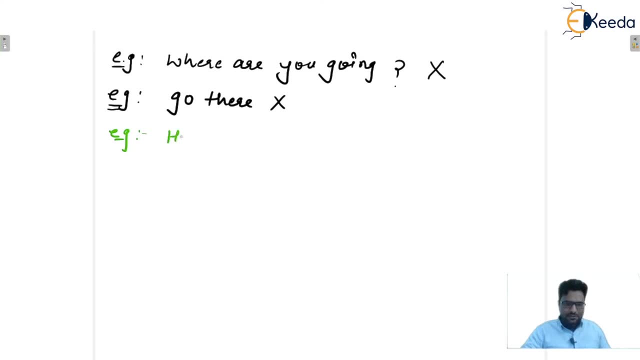 to exclamation. let us consider how exciting. now you only tell me how exciting. this one is, neither true nor false. so we can say that this one is also not a proposition, yes or no. so i hope this one is clear to everyone. so you can write down one note. yes, write down one note in note. you can write down. 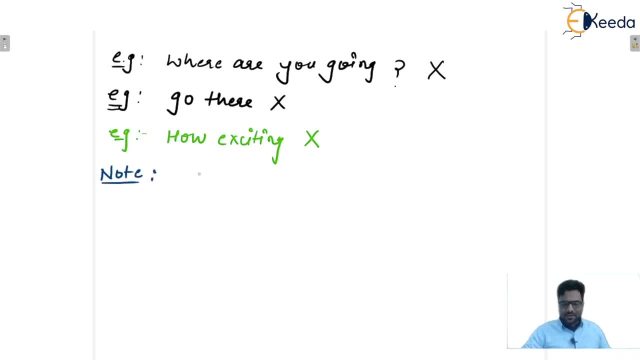 first, yes, we can say that questions, exclamations and commands are not propositions. so write down one note: we can say that questions, exclamations and commands are not propositions, isn't it? i hope this one is clear to everyone: questions, exclamations and commands are not propositions. 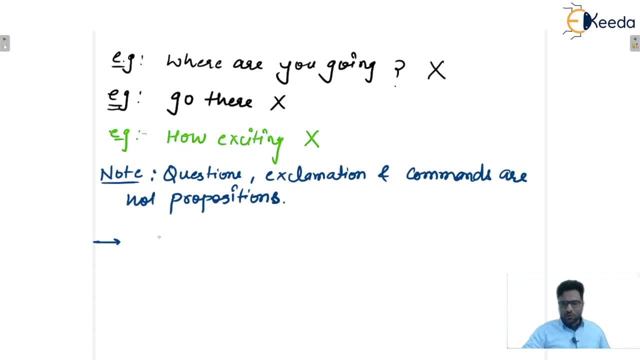 okay, next one you can write down: yes, we will use some variables to represent any proposition. so let's say p, q, r, s and so on. we can say that these type of variables are used to represent any proposition. okay, so we'll see. yes, these letters are used to denote. 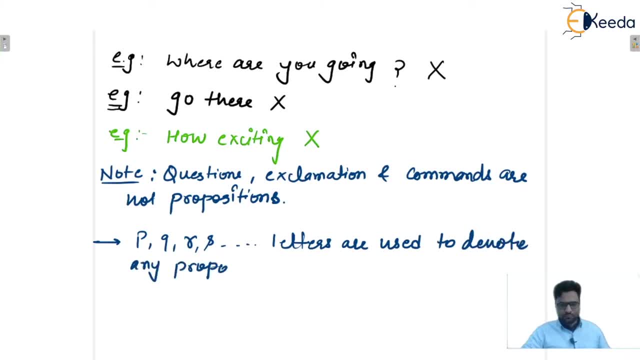 any proposition, isn't it? and these are what these are: propositions, proposed propositional variables. okay, any letter, english letter, is used to denote the proposition and that will be known as propositional variable, isn't it? i hope this one is clear to everyone, okay? so next one is: yes, we can say that next statement is what we can say that next? 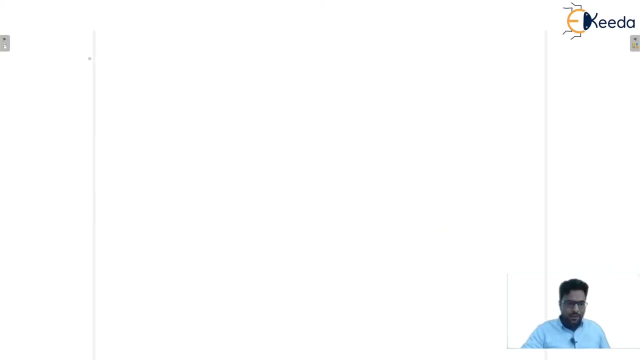 one is yes. we can say that next one is your propositional logic. so we'll see what's our next statement. yes, i'll do that only for one وا. so next one is yes. we can say that next one is togetherGet. one way to another, one way to. 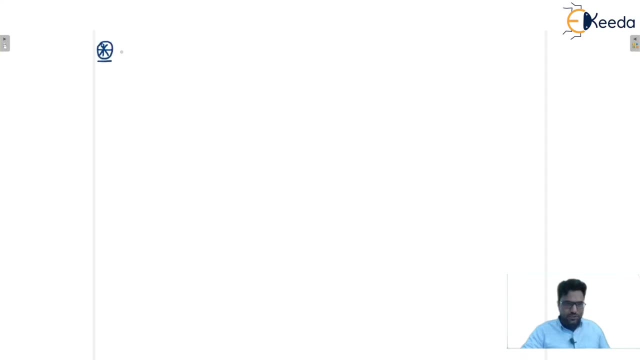 predict your proposal. another one way to можете. other one way to predict your proposal. okay, we'll see another way to what is propositional logic or propositional calculus. We will see what is propositional logic, or it is also known as propositional calculus, So we can say that the area of logic. 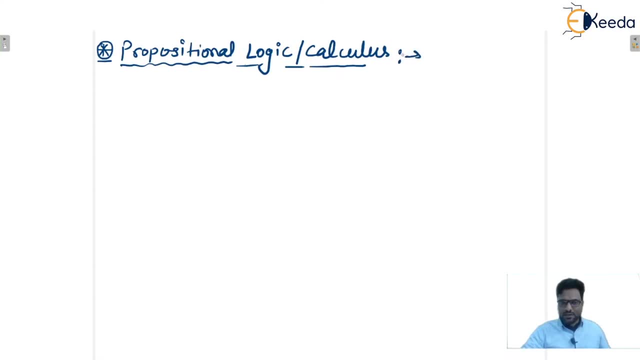 that deals with propositions is known as what Propositional logic. So write down, yes, write down the statement. The area of logic we can say that deals with propositions is called as we can say, that is called as propositional logic. Okay, Okay, guys, I hope this one is clear to. 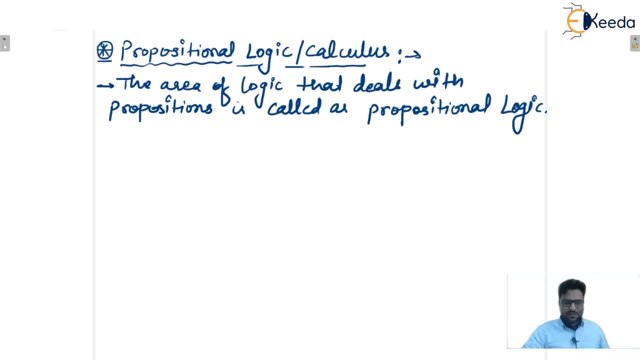 everyone. What is proposition Okay? Next one, we'll see. Yes, some. we can say that logical connectives. So logical connectives are. we can say that operators which are used to connect the logical statements. that is proposition Okay, So logical. 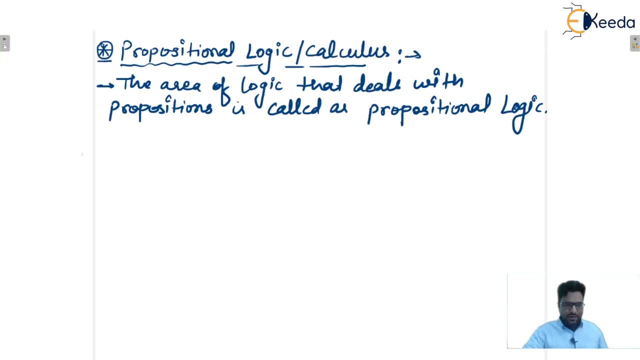 connectives are used to connect the proposition. Okay, So our next topic is what we can say that logical connectives. Second one is logical connectives. So we can say that these connectives are used to connect the propositions. Okay, So our next topic is what we can say that logical. 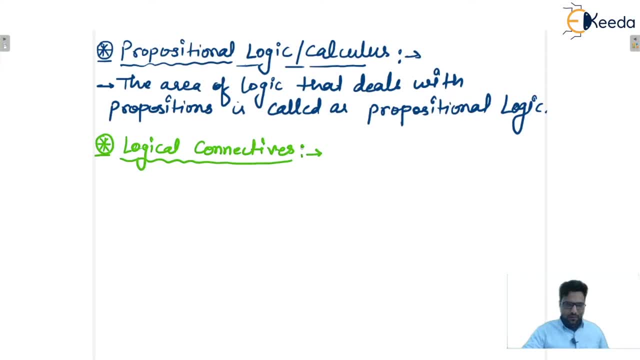 are used to connect the yes propositions. First one, we will see what is negation. after that we will see the logical connectives. So, negation of a proposition P, proposition P that is denoted by this particular sign that is negation P, or this tilted sign that is used to represent the negation. 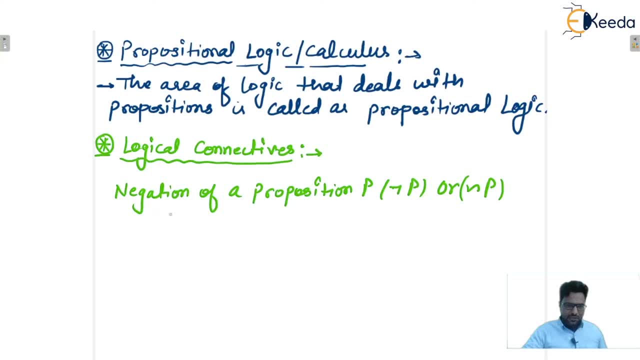 of P, Isn't it? So we can say that negation of a proposition: P is what In English statement we can write down it like that. It is not the case. It is not the case that P That is the negation. 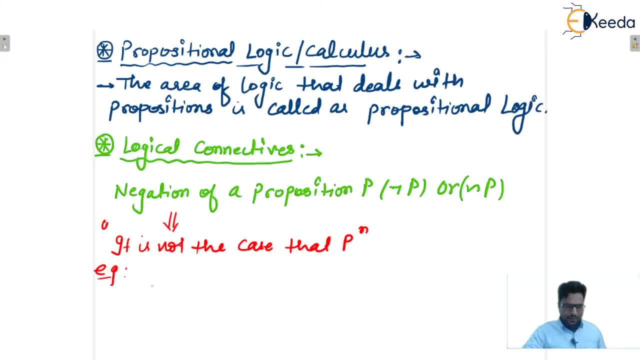 So consider one example. Let us consider one example. Let's say one proposition. today is Friday, Today is Friday. So yes, this one is a proposition or not. Yes, this one is a proposition. Either it will be true or false. So what will be the negation of this statement? You only tell me, So we can say that. 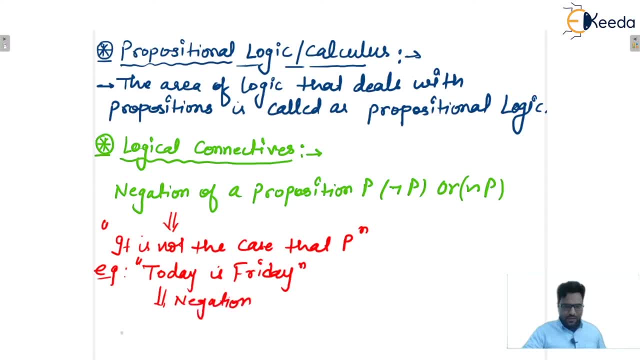 negation of this statement will be what We can say: that it is not the case that today is Friday. It is not the case that today is Friday, Isn't it? Or, simply, we can say that today is not Friday. Today is not Friday, Yes or no. Simply, it is the negation. So we will see what is the truth table. 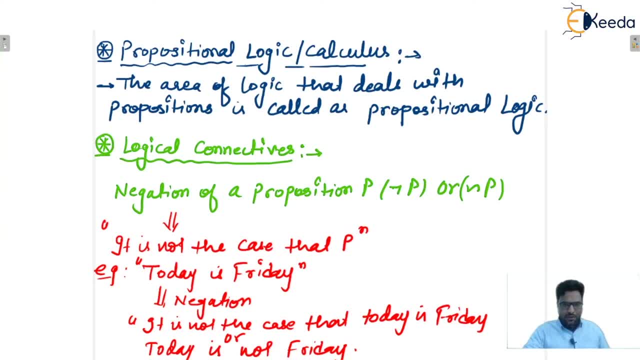 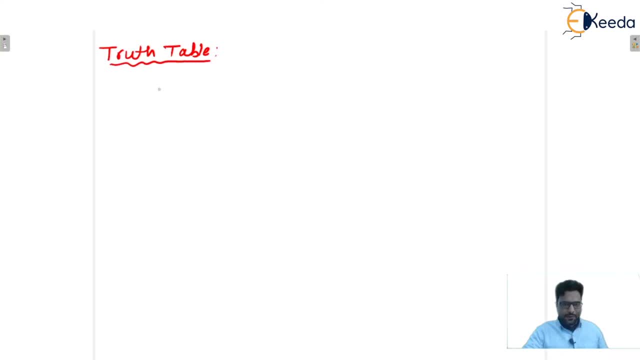 of negation. Okay, So write down next Truth table of negation operator So we can see. Let us consider one variable, Propositional variable. Let us say P. Yes, if it is one variable, or that means one proposition, then it can take two values. That is true or false. So if P is true, then negation P will be false. 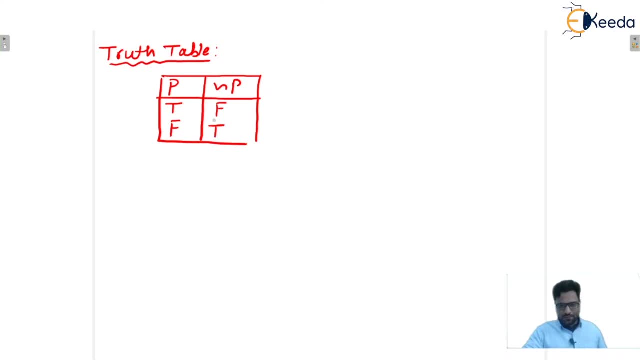 and P is false, then it will be true, only Isn't it. That's why we can say that negation of true is what False, and negation of false will be true only. That is the truth table. Okay, Write down first one Logical connectivity. 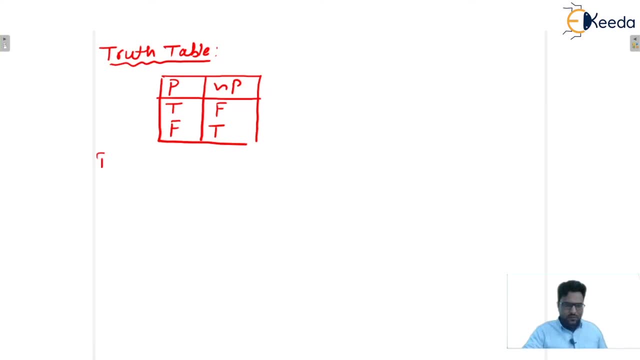 Yes, Under the logical connectives write down first one. That is, we can say that let us consider P and Q are two propositions, Then first one is P and Q. P and Q- this operator is known as what Logical and or it is also known as conjunction. So we can say that this: 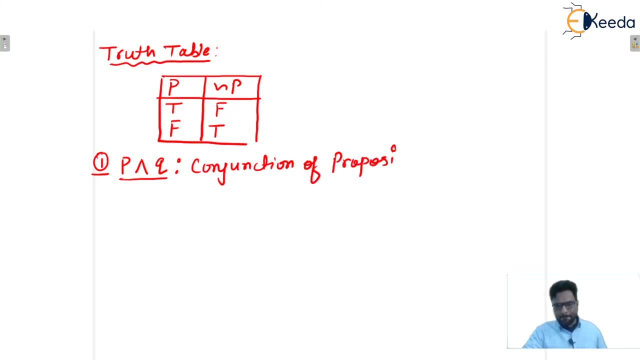 is conjunction of proposition P with. we can say that proposition Q- And you only tell me this one- is true when, when both P and Q are true, So we can say that P and Q is true. It is true when we can say that both P and Q are true, Okay And false. 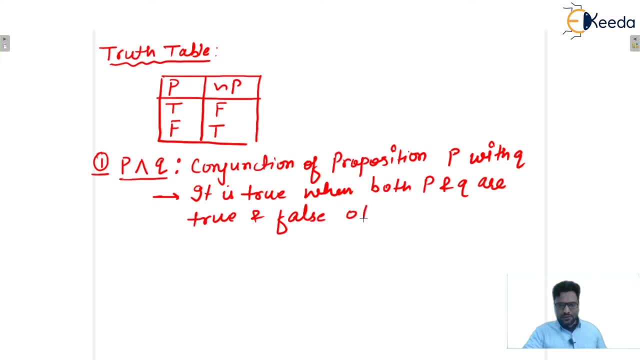 otherwise And false otherwise, Isn't it? I hope this one is clear to you, Okay. So, yes, we will see the truth table. Yes, what will be the truth table? You only tell me, Yes, there are two propositions, let us say P and Q. So with two, 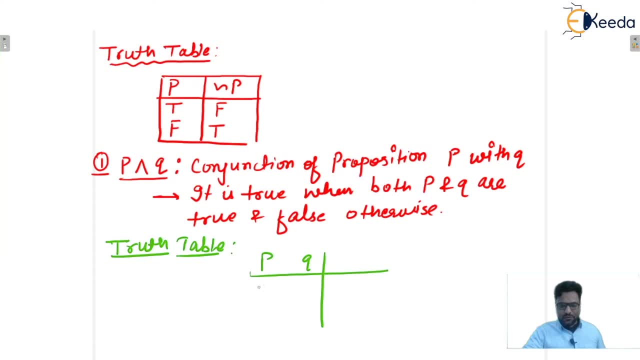 propositional variables. we can say that four possibilities or four combinations are there. These can be true, true, Then we can say that true, false, Then false, true and last one is false, false. So what will be the truth? value of P and Q. 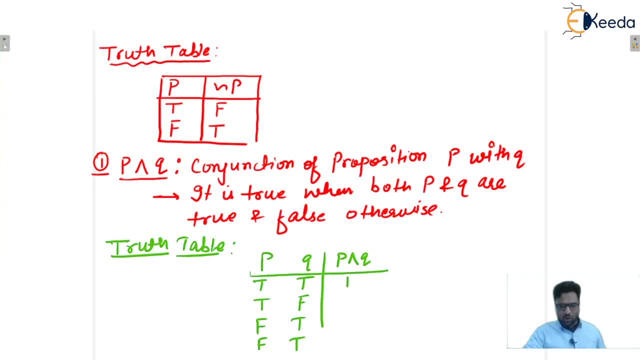 You only tell me Yes, truth value of P and Q will be true only, Yes or no, Because both are true. Here we can say that P is true but Q is false. Because of that, this one will be the false only, and this one will be the false only, and this one will be the false only. That will be the truth. 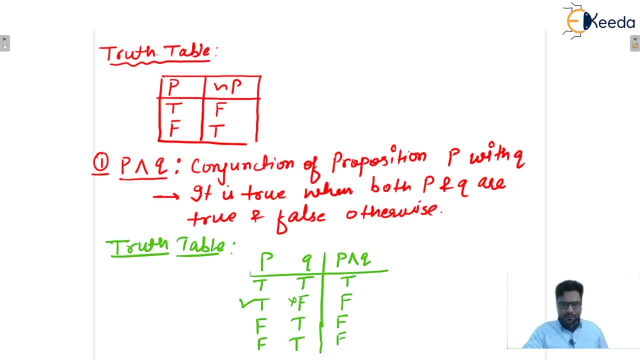 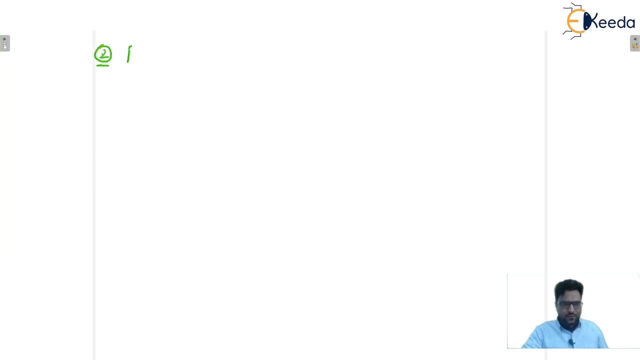 table. I hope this one is clear to everyone. Okay, Right now. next one: that is your P or Q. Next operator or logical operator, Next operator or logical operator, Next operator or logical connectives. That is P or Q, This or logical, or is also known as disjunction. 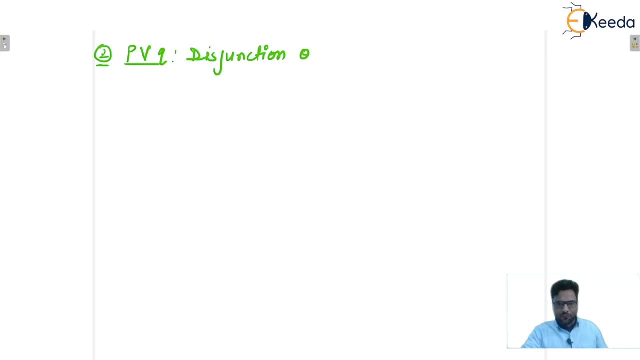 So we can say that this is a disjunction of proposition P, Disjunction of proposition P with. we can say that proposition Q Isn't it? Yes? So right now, next point, we can say that this one is false. We can say that it is false. 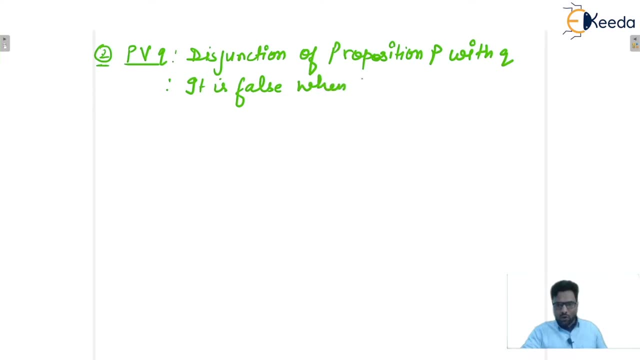 When both variables are, yes, false, only Then it is false and we can say that true, otherwise, Yes or no. Or we can say that true, otherwise, Yes or no. So if we see the truth table, Yes, you can see What will be the truth table, Yes or no. So if we see the truth table, Yes, you can see What will be the truth table. 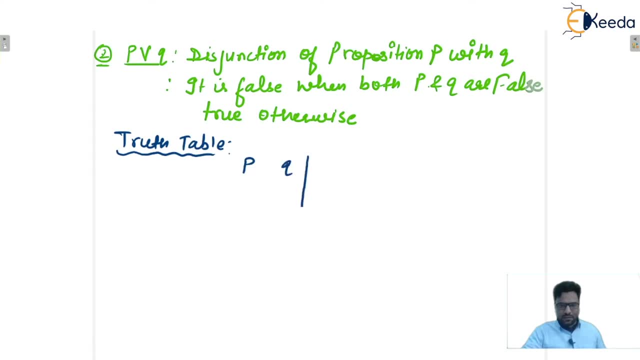 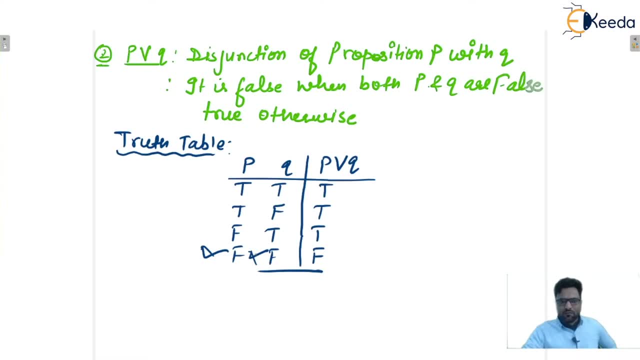 values, Isn't it? So we can say that this one will be the truth table of P or Q. Okay, Okay, Moving to the next one, that is your XOR operation, Isn't it? Third one is XOR, So write down next. 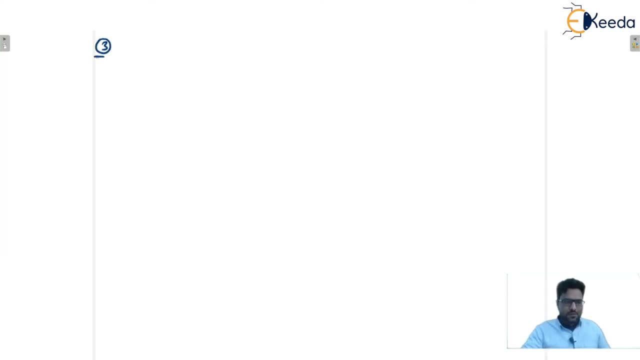 one Third one. this one is your P exclusive OR with Q, Yes or no. So we can say that let's say P and Q are the propositions. then we can say that this one is what: P exclusive OR with Q, Yes or. 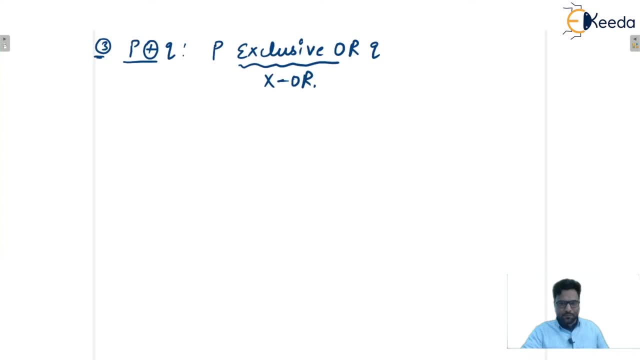 no, Or simply it is also written like this: XOR operation. So in English statement it is written like that: either P, either P or Q, but not both. Either P or Q, but not both. That is known as yes P, XOR Q, Isn't it So? meaning is what? This one is true. Yes, 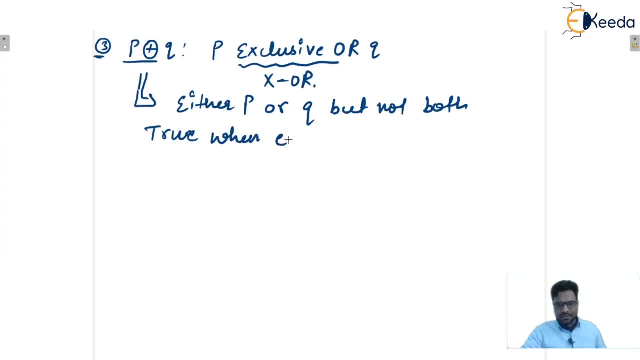 we can say that when exactly one out of P and Q is true, Then only we can say that the truth value will be the true, Otherwise false. Otherwise it is false, Isn't it? So let us take the yes. Have a look at the truth. table of P, exclusive OR. 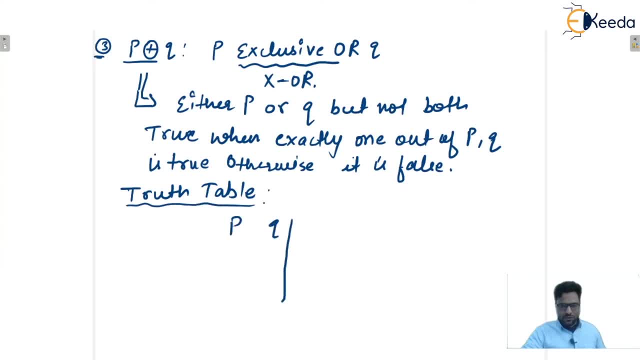 with Q. So let's say two variables, propositional variables, P and Q, and this is the exclusive OR operation. So four combinations are possible: True, true, True, false. Then we can say that false, true and false, false, So this one will be the true. 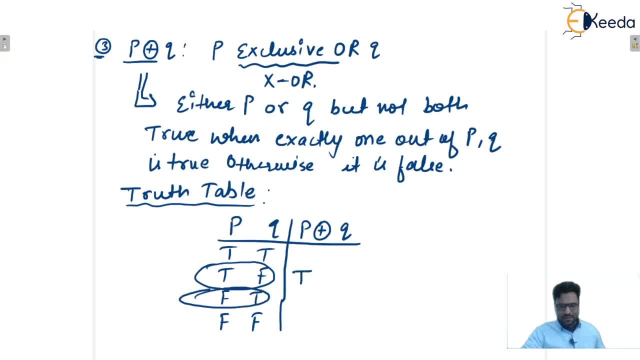 Exactly, one is true. That means this is true. Yes, this one is also true. and in this case, first one, true, true, This one will be the false, and in last one also, it will be false, only, Isn't it Okay? So these were some basic logical connectives. Now we will see. 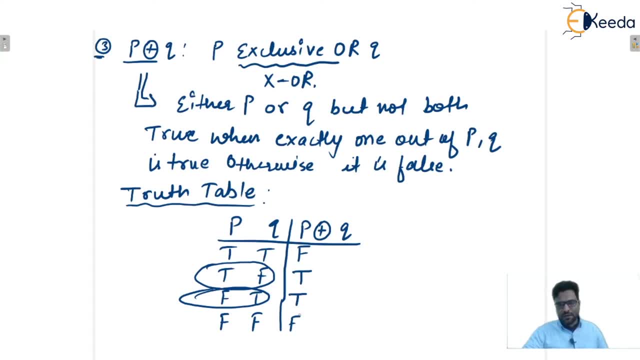 some conditional statements which are very, very useful in mathematical logic. Okay, So, whatever portion we will cover In the next videos, So here, everywhere you will see the importance of conditional statements, Okay, So our next topic is conditional statements only. that is very, very important, in which? 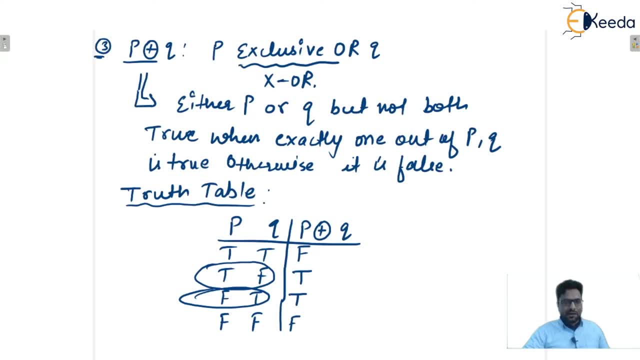 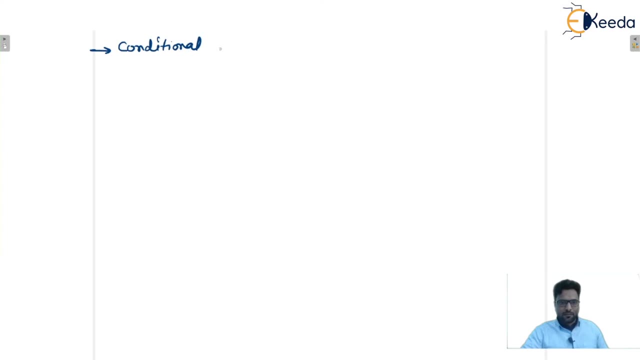 we will see. what is P implies Q, what is P by conditional Q, and so on, Isn't it? Okay? So these two conditional statements are very, very important. Okay, So next one is: our topic is conditional statements. Conditional statements: Okay, We will see. Yes, we can say that. we will discuss, yes, several. 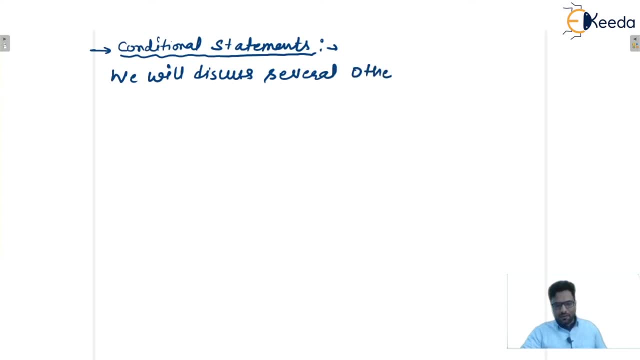 we can say that other important ways, several other important ways in which we can say that propositions can be combined, okay, okay, and that will be combined with conditional statements, okay, Okay. So first one we will see: P implies Q. this arrow sign is implication. 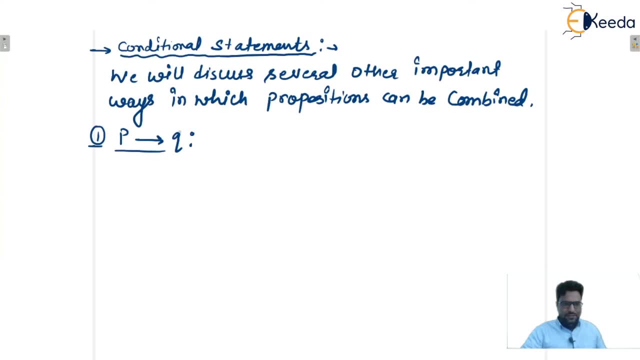 for we will call it like a P implies Q or this is the implication sign. So we can say that yes, can say that yes, this statement is, is known as what we can say, that implication, and we can say that this conditional statement, this conditional statement- why it is called conditional? because 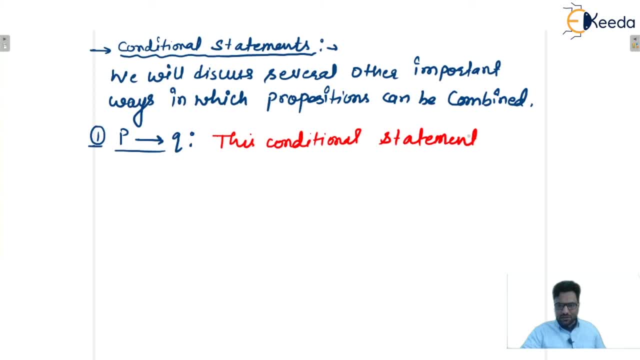 one condition is associated. okay, we'll see what is the condition. this conditional statement p implies q. yes, we can say that is the proposition. yes, we can say that is the proposition. remember, guys, p and q, these are also propositions, isn't it? so p and q are the propositions. 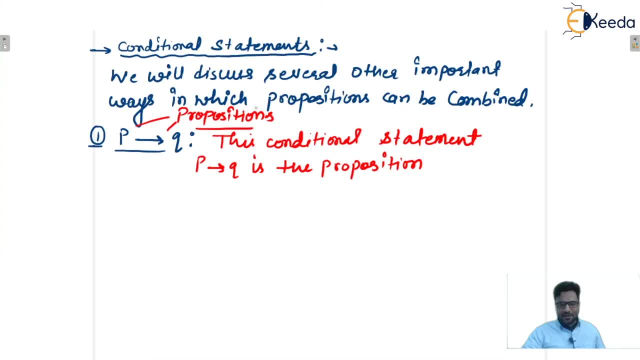 so we'll see this conditional statement: p implies q is also the proposition. and what is the proposition? yes, that is a represented or denoted like that. you, if p, then q isn't it. that is the yes conditional statement and it is also a proposition. okay, so we. 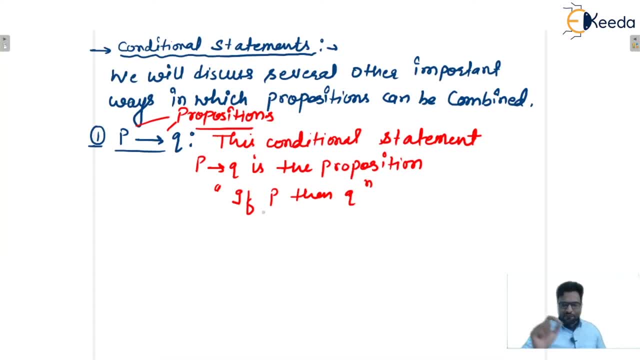 can say that the meaning of this one is what: if p is true, then q must be true. then this particular implication will be the true, isn't it otherwise? yes, we can say that if p is true and q is false, then the truth will be true, and if p is true, then q is false, then the truth will be true. 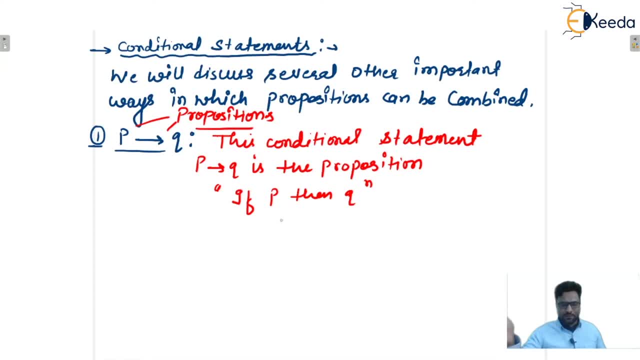 value of this implication will be false, only isn't it clear. okay, guys. so we can say that, yes, we can say that this conditional statement is false, it is false. we can say that when p is true and q is false, it is true otherwise. so remember, guys, this one is very, very important. yes, we can say that p implies q is false. yes, this, 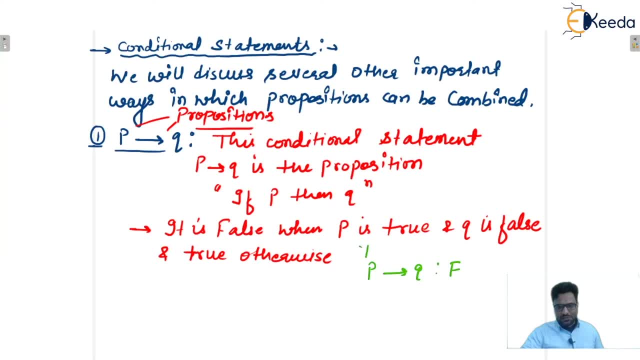 one will be false. when yes, p is true and q is false means left hand side is true and right hand side is false, then only the truth value of this implication will be false. otherwise it will be true only okay. so in p implies q. we can say that yes, if we take the or if we design the truth. 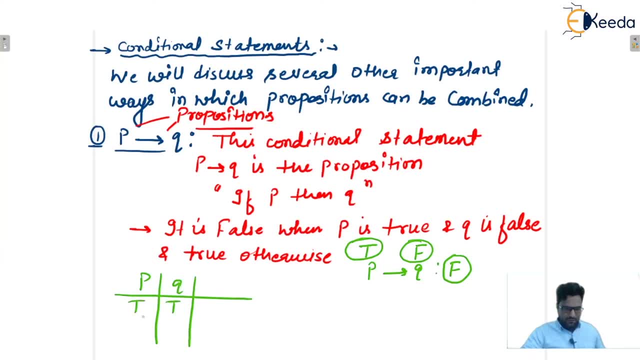 table. then we can say that there are four possibilities: yes or no. there are four possibilities. out of these four possibilities, we can say that this one will be the false only in one case, when p is true and q is false. so it is false and true, otherwise yes or no. also remember, guys: 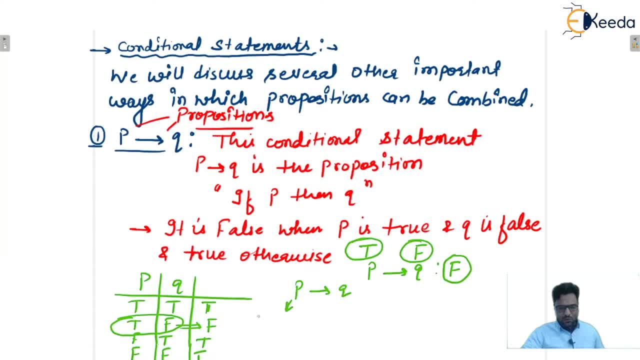 in p implies q. this left hand side is also known as hypothesis and rhs is known as what we can say, that conclusion, or we can say that consequence isn't it. and left hand side is called as what we can say that hypothesis or antecedent, or we can say that premise Isn't it Okay? 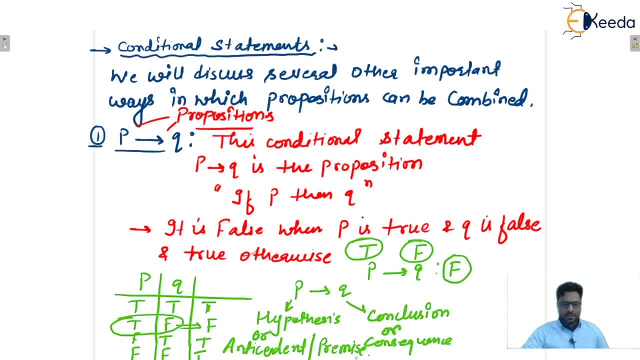 So we can say that that is P, implies key 2.. So, guys, we will see a variety of terminologies are used to express this implication. Okay, And the meaning of these old terminologies will be the same. only So we will see, one by one. Okay, So we can say that, yes, you only. 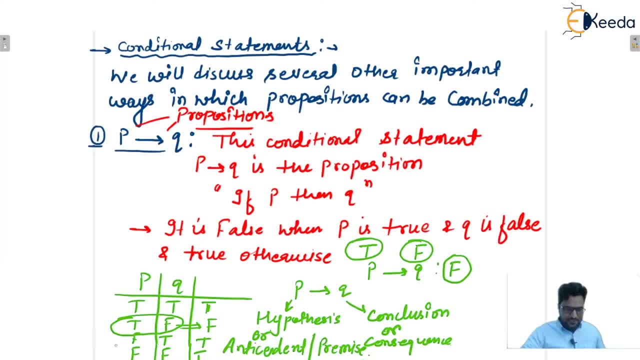 tell me yes. here only we can say that if P is false, you only tell me yes, you only tell me by observing the truth table. you only tell me: if P is false, then whatever be the value of Q, the truth value will remain 2 only. Yes or no. So we can say that in P implies Q if 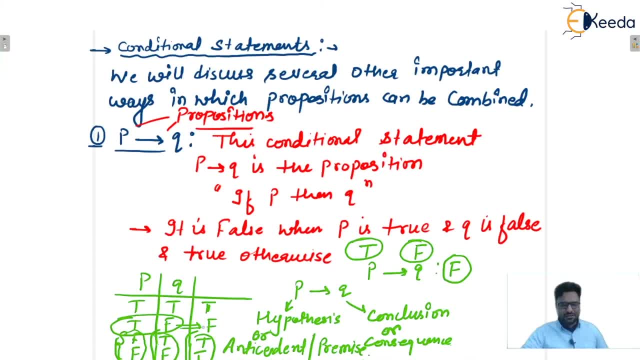 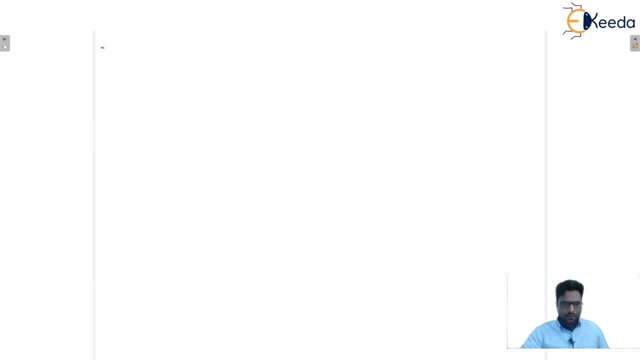 P is false, then whatever be the value of Q, either It is true or false. final truth value will be the true, only Isn't it Okay. So we will see variety of terminologies which are used to express this yes implication. So write: 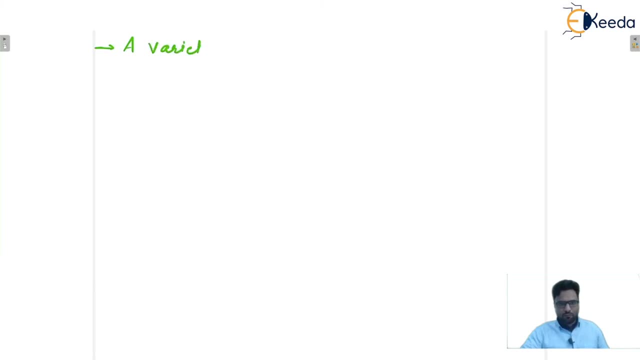 down a variety of- we can say that terminologies are used. we can say that to express yes, P implies Q, So we will see one by one. Okay, Okay, guys, Okay, I hope this one is clear to you, First one we will see. this one can be written like this: Yes, you only know, this is also yes, we. 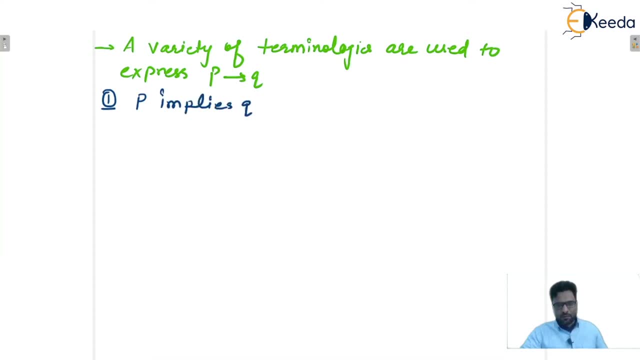 can say that this one is P implies Q. Second one: it is also represented like this Second one. we will see: yes, if P, yes, we can say that, then Q meaning is same. that is, P implies Q. Yes, we can say that this one is also P implies Q, Isn't it Next one? yes, we can say that. third, 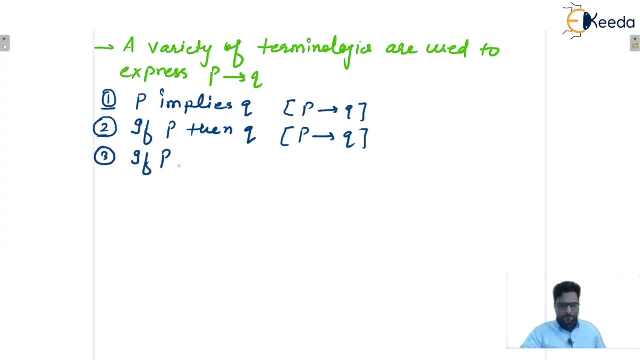 one, it is also written like this: if P, comma, Q, Yes, meaning is same, that is, P implies Q. Also, it is written like this: yes Q. if P- Yes, meaning is same, that is P implies Q. Next one: it can also be written like this: 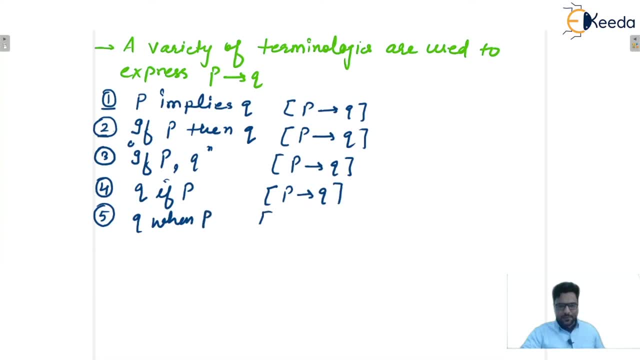 Q when P meaning is same. that is, P implies Q. Okay, Also, it is written like that. Sixth one: Q whenever P, whenever P. the meaning is same. that is, P implies Q, Isn't it? Next one, yes, it is also written like this: Q follows from P, Isn't it? The meaning is same, that. 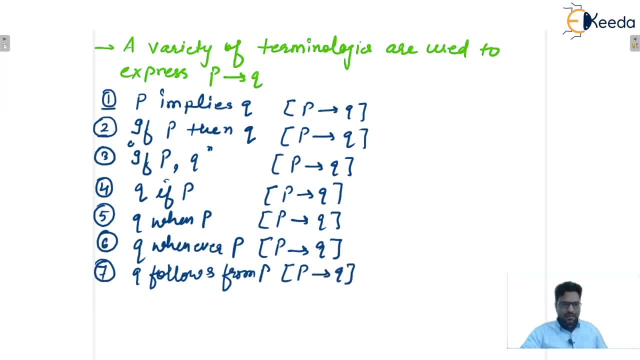 is: P implies Q. Yes, we can see next one, that is eighth one. Yes, it is also written like that. we can say that P is sufficient for Q. P is sufficient for Q meaning is what P implies Q, Next one. we can say that ninth one: yes, Q is necessary, for. we can say that P meaning is same, that 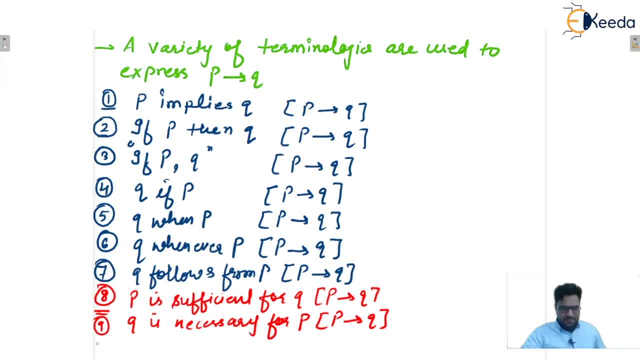 is P implies Q. Next one: we can say that tenth one, that is Q, unless negation P Meaning is same. that is, we can say that P implies Q. And eleventh one: we can see eleventh one is P only if Q, Isn't it. So remember guys, first seven: you know very well These one are very. 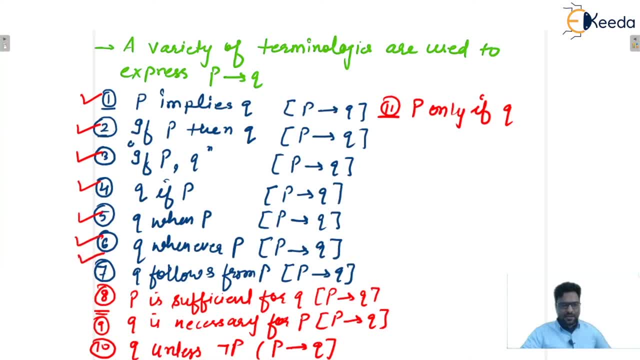 simple one. Yes, you know. Yes, meaning is same, that is, P implies Q, But the problem is where we can say that. the problem is in the eighth, ninth, tenth and we can say that eleventh. So you will see, Yes, you want to know why it is known as P is sufficient for Q and why. 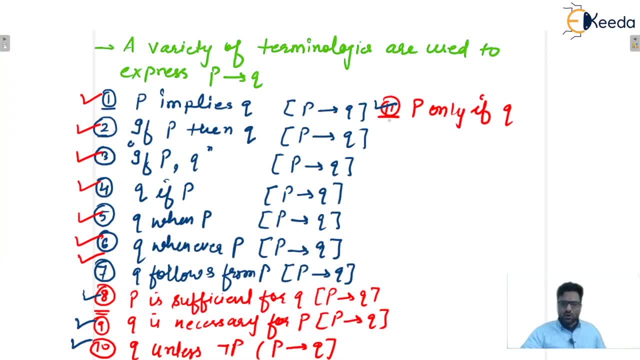 it is called Q is necessary for P and why it is called Q unless negation P, and why it is P only if Q- Remember, Remember guys, this one- is only if. then we can say that the meaning is P implies Q, And if it is, or we can say that if only is missing, then it becomes P, if Q, then the meaning will. 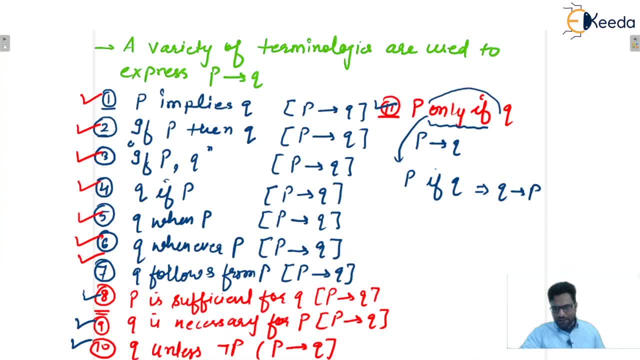 be what Q implies P, But if it is- only if, then the meaning is implication, Isn't it? I hope this one is clear to everyone, So I will discuss these points: eighth, ninth, tenth and eleventh. Isn't it Why it is Yes, equivalent to P implies Q. Okay, So let me see once. 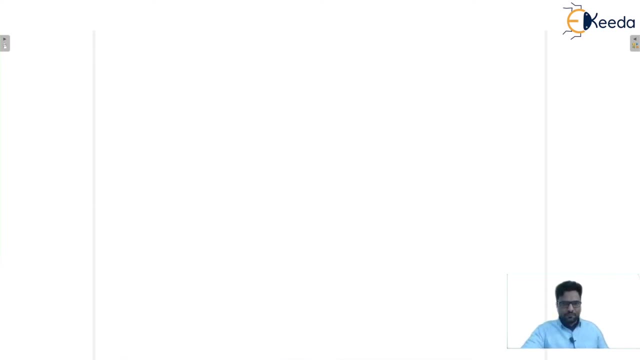 Okay, So first one, we will see: Yes, Yes. first one we will see: P is sufficient for Q. That is equivalent to Yes, P implies Q, Yes, we can say that, for example. let us consider one example: Yes, So you only tell me. yes, this one is clear to everyone, or not? For example, we can say: 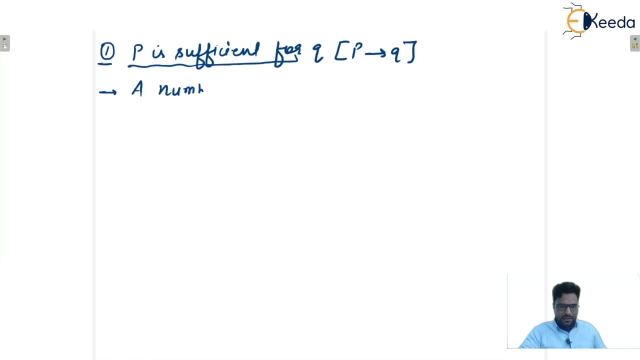 that a number, Yes, we can say that a number being divisible, Being divisible by four, Yes, is what we can say. that is sufficient but not necessary. Yes or not? Yes for it to be even, Isn't it? So we can conclude that, yes, if it is equivalent to P implies Q. then we can. 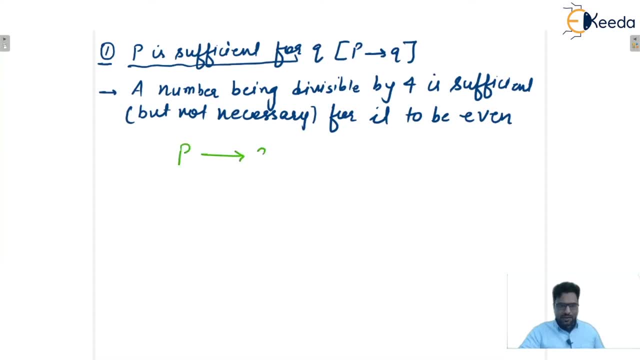 consider or we can write in logical statement like that: P implies Q, where P is what. we can say: that a number being divisible by 4.. Isn't it divisible by 4? and Q can be written like that: it is even Yes or no. So we can say that if a number is divisible by 4, then it will be the. 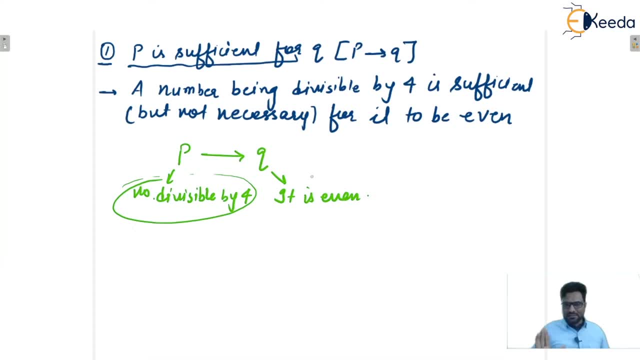 even number, Yes or no? Yes, Isn't it? If a number is divisible by 4, then we can say that it is even. but we cannot say in reverse manner, that if a number is even, then it is divisible by 4.. We cannot say like that: Yes or no. 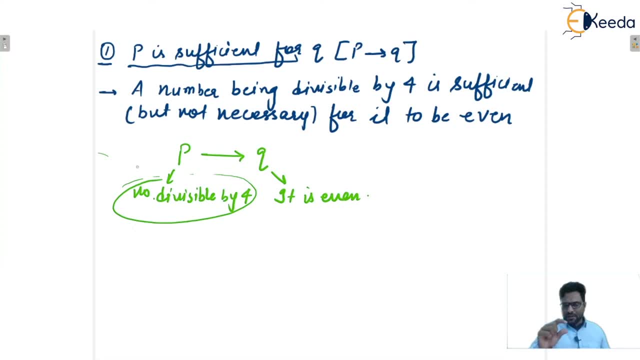 Yes or no, But left to right. we can say that yes or no. If a number is divisible by 4, then it is even Yes or no, That is true. But we cannot say that if a number is even, then it is divisible by 4.. No, We cannot say So. we can say that a number being divisible by 4 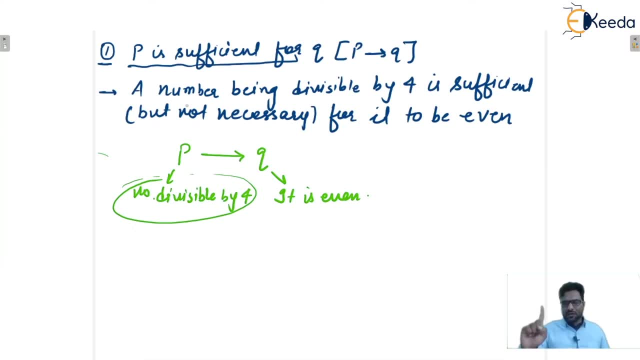 is sufficient, but not necessary for it to be even. That's why we can say that this P- yes, we can say that P is sufficient. Sufficient for Q is equivalent to P implies Q, Isn't it? I hope this one is clear to everyone. 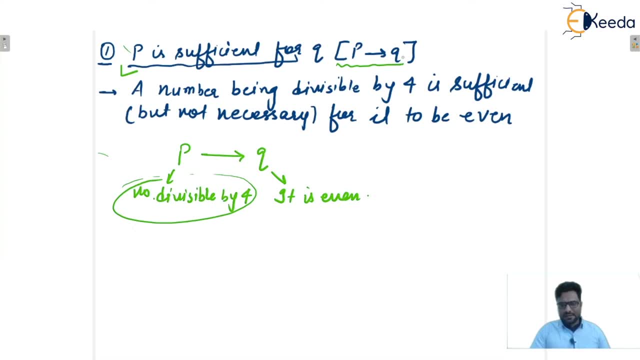 or not? Okay, Yes, So we can say that this one is yes. P is sufficient for Q. Next one: let us take one more example. Let's say: yes, we can say that John is a king implies we can say that John is male, Isn't it? So we can say that here, knowing that John is king, we can say: 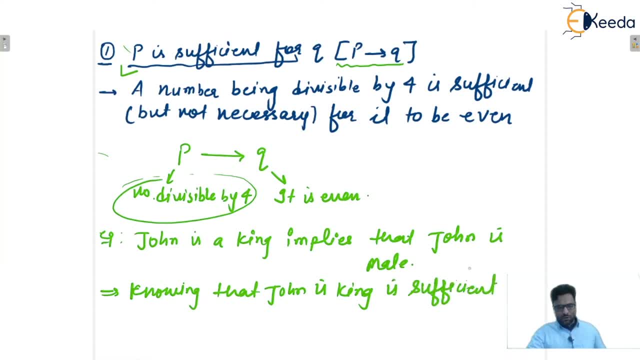 that is a sufficient to know that he is male, Yes or no. Similarly, we can say that from here we can conclude that John is male- is necessary condition. we can say that for John to be a king, Yes or no, So we can say that this statement can be called like that. This is implies. implies means: this one is P. Implication sign is this one. this one is Q. So we can say that John is a king implies John is a yes, male. 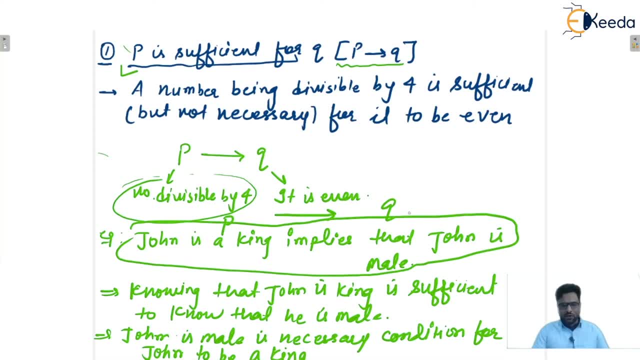 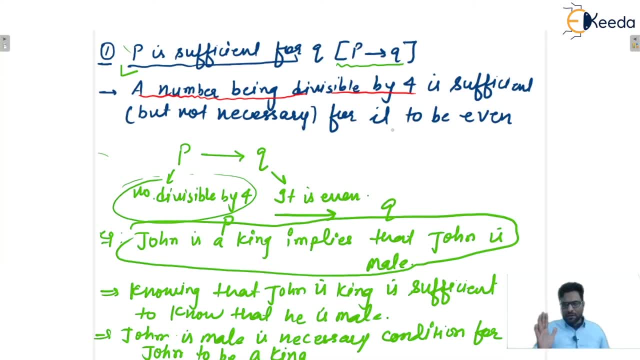 say that yes for 2, for it to be even number is a necessary condition if it is divisible by 4.. Yes or no? So we can say that if it is divisible by 4, then we can say that it will be even, but in 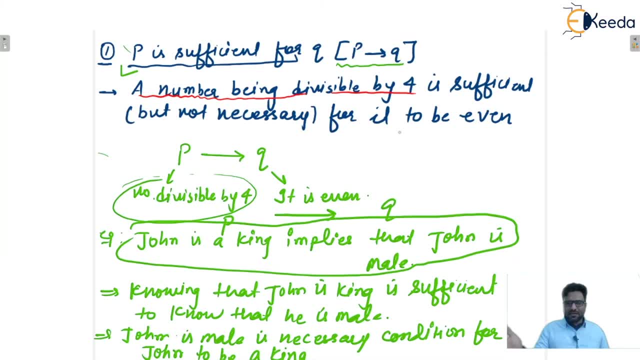 reverse. we cannot say that if it is even, then it is divisible by 4, because it can be divisible by 2 also, Isn't it Okay? That's why we can say that yes. similarly, we can say that here Q is necessary for yes, we can say that necessary for P. meaning is same, that is, P implies Q, Q is necessary means: 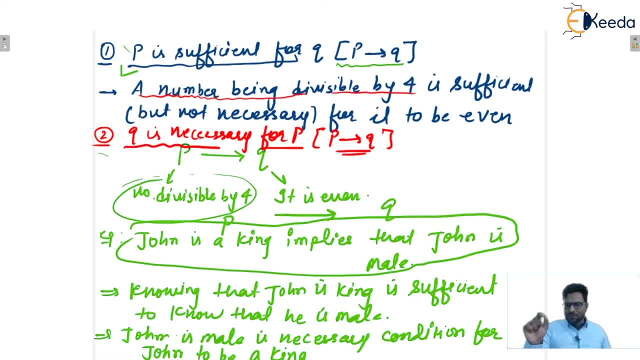 means if it is divisible by 4, then necessarily it will be even Yes or no, Isn't it Okay? I hope this, This one, is clear to everyone. So next one will proceed to yes. next one will see why. P only if 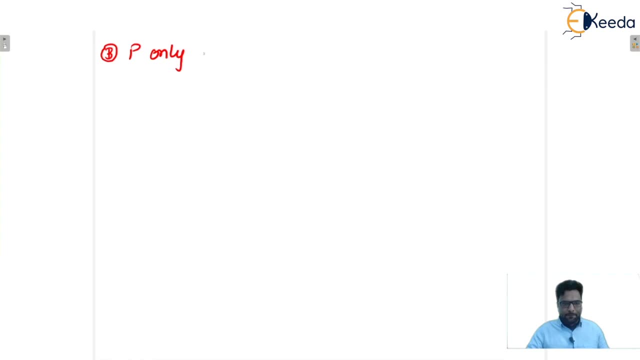 third one is equivalent to P, implies Q. So we can say that P only if Q. This implies, we can say that this one is equivalent to P, implies Q, Why? Yes, I am explaining this one. You can observe that P only if Q means what. We can say that P is true only if Q. 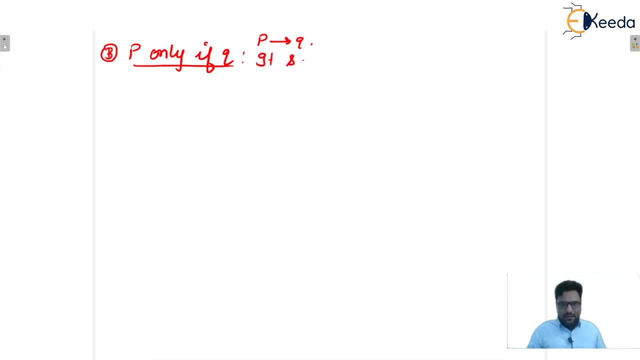 If Q is true, That means it says what We can say that it says that yes, P cannot be true, Yes. when we can say that Q is not true, Yes or no, That means what That is. we can say that the meaning is what That is. we can say that the statement is false when. 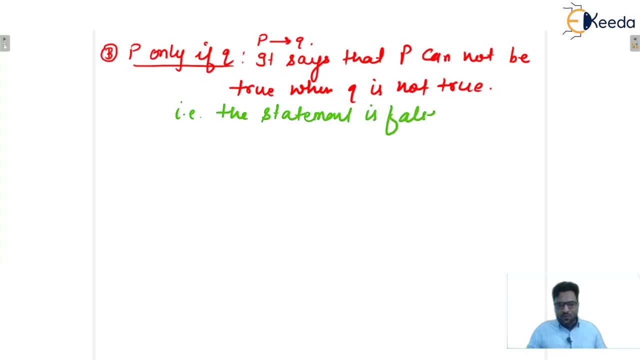 the statement is false when, Yes, we can say that if P is true and Q is false, Yes or no. And yes, if P is true and Q is false, then the statement is false. then the meaning of this one is what We can say: that P implies Q only. That's why we can say that P, only if Q is equivalent to P, implies Q. 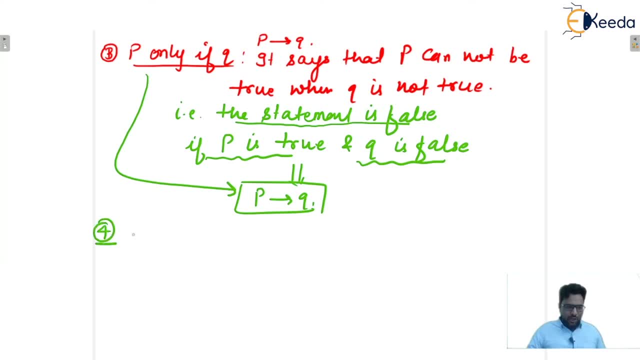 Next one, Yes, last one. We can say that Q unless negation P, unless means yes, except. so meaning is what we can say: that Q is true except negation P is true, yes or no. so meaning is what we can say: that it says what it says. 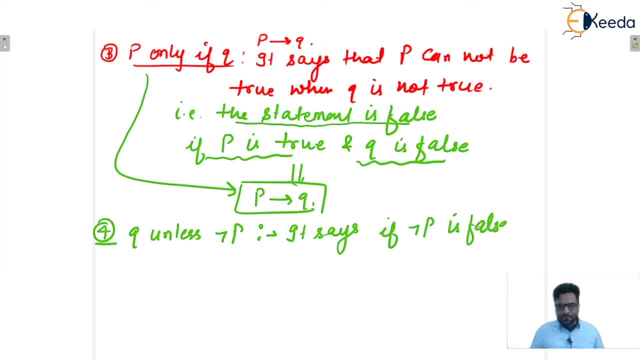 if negation P is false- yes, we can say that- then, yes, we can say that Q must be true, isn't it? I hope this one is clear to your knowledge so we can say that it says: if negation P is false, then Q must be true, yes or no, isn't it? so meaning is, what we can say, that the statement is false. 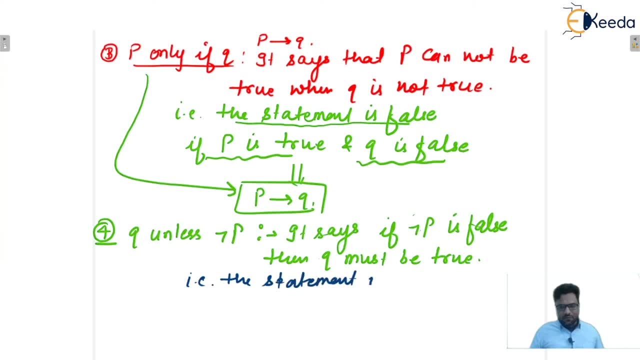 we can say that the statement is false. we can say that, yes, when negation P is false, negation P is false and we can say that Q is also false, yes or no, then this statement will be false. only we can say that if negation P is false and Q is also false, then this statement will be false. 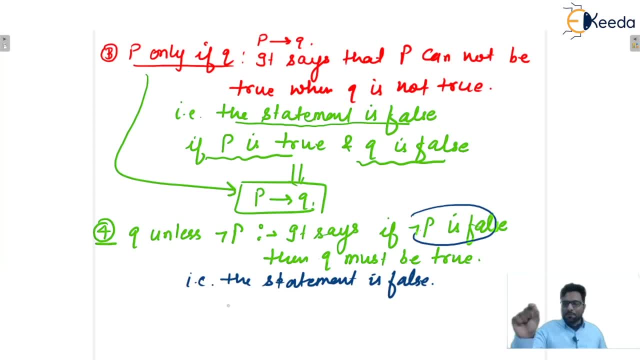 so negation P is false means P is what. P is true, yes or no. so we can say that when yes, negation P is false means P is true, because negation of true will be false. only P is true. that means negation P is false. and we can say that Q is false, yes or no. so we can say that this statement is false when 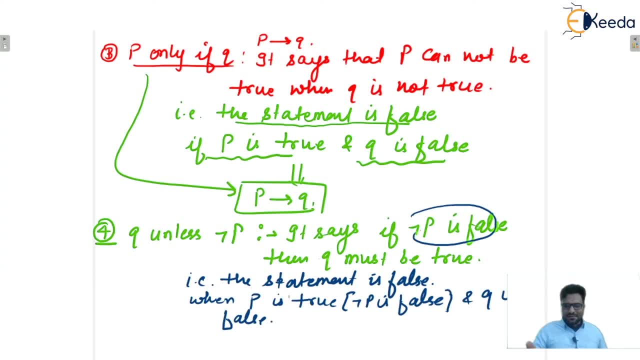 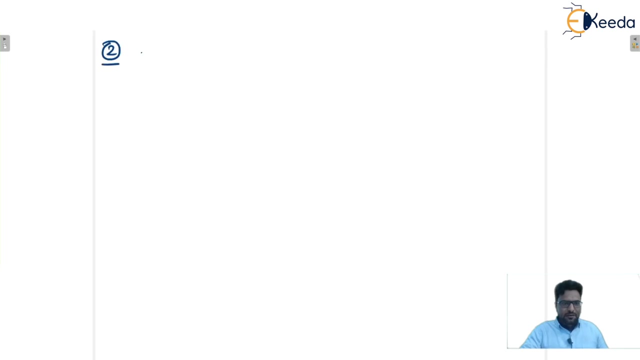 when P is true and Q is false, and this happens in the case of P implies Q. only that's why we can say that Q, unless negation P is equivalent to P, implies Q. I hope this one is clear to everyone, okay. so last one, we'll see. yes, that is your yes. second conditional statement that is known as: 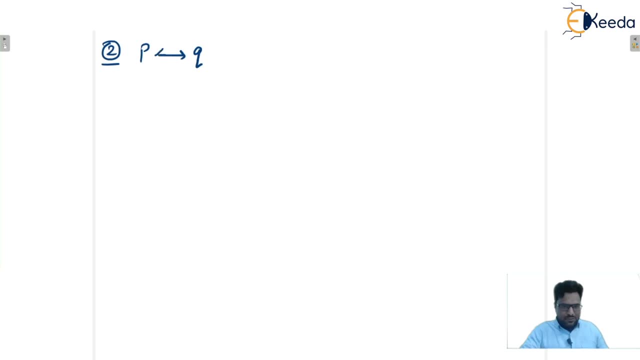 P biconditional, that is, P implies Q as well as Q is false. so we can say that Q is false, P implies P. that is known as what the biconditional statement and meaning is what we can see. biconditional statement: yes, we can say that. yes, P biconditional Q is what we can say. that. 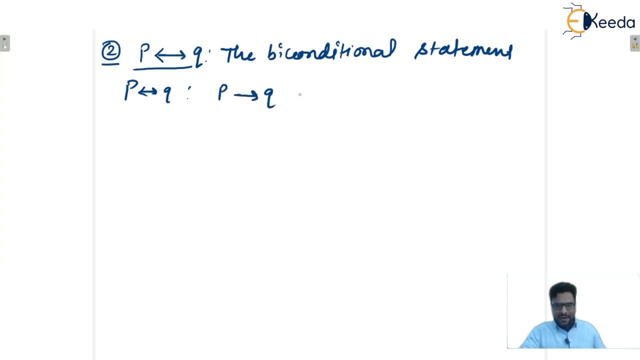 yes, P implies Q and this is logical and we can say that Q implies P also. so if we say that Q is false, then we can say that Q is false, and we can say that Q is false if we see the truth table of this one, so we can say that this one will be what. let's say these are: 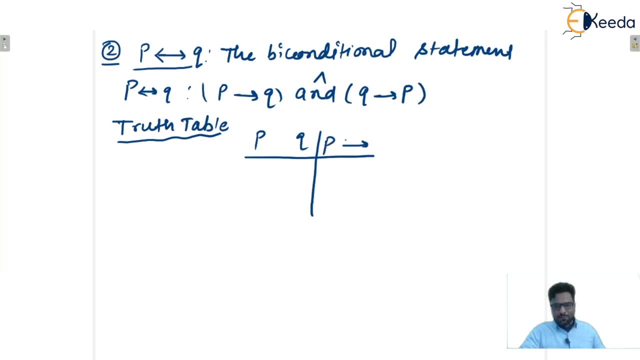 the P and Q two variables, and this is P biconditional Q. so four combinations are possible: true, true, true, false. then we can say that, false, true and last one, false, false. so we can say that in true, true, it is true only. but because of P implies Q, yes, here it will be false. 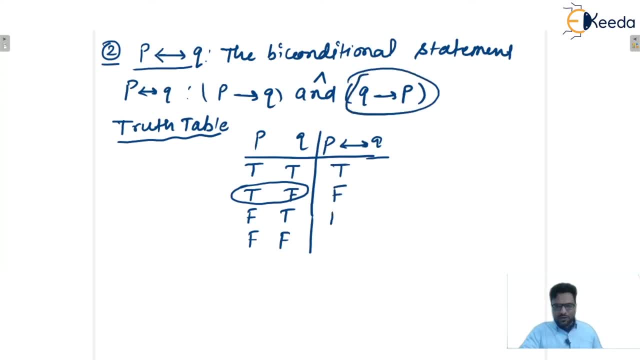 and because of Q implies P. here also it will be false, yes or no, and in case of false, false it will be true. only isn't it because Q implies P will be false when Q is true and P is false. that is your third combination, isn't it? I hope this one is clear to everyone, or not? 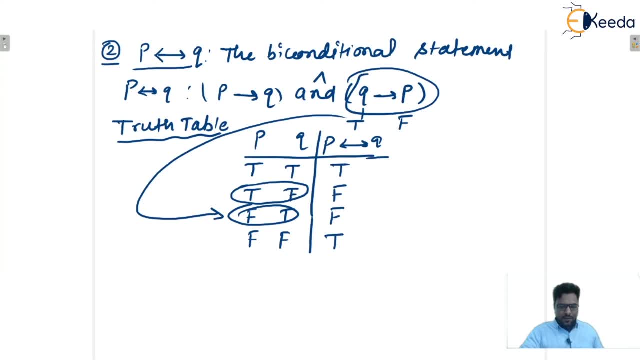 okay. so we can say that yes, you only tell me. yes, we can say that P, biconditional Q, yes, can be expressed by Q and P is false. so we can say that, yes, we can say that P is false can be expressed as we can say that first one. we can say that it is also yes, sir, represented. 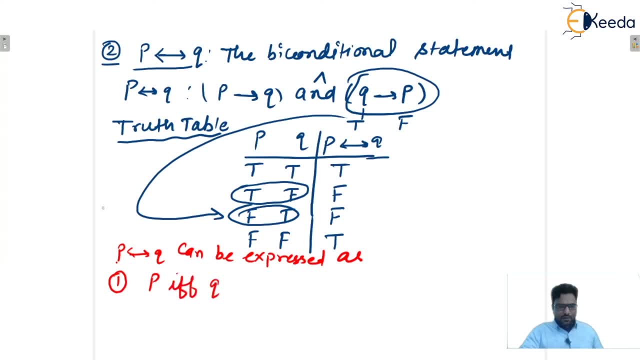 like this: P, if and only if Q. this one is what we can say, that I double F means if and only, isn't it okay? also, it is written like this: P- biconditional Q. also, it is also written like this: P implies Q as well as, and means as well as, or logical and negation. yes, Q implies P. 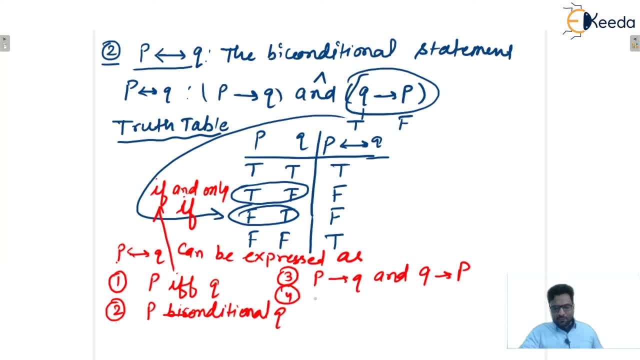 and fourth one. we can write it like that or not. you only tell me P is sufficient for Q, yes or no? for because of P implies Q, we can say that P is sufficient for Q, and because of Q implies P, we can say that P is necessary for Q. So we can say that P is sufficient. 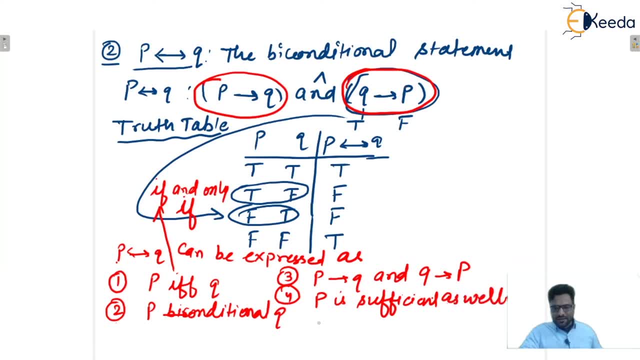 as well as yes, we can say that necessary for Q, Isn't it? P is sufficient as well as necessary for Q. Also, we can say that Q is sufficient as well as necessary for P. I hope this one is clear to everyone, or not? Okay, So that is the biconditional. This means left to. 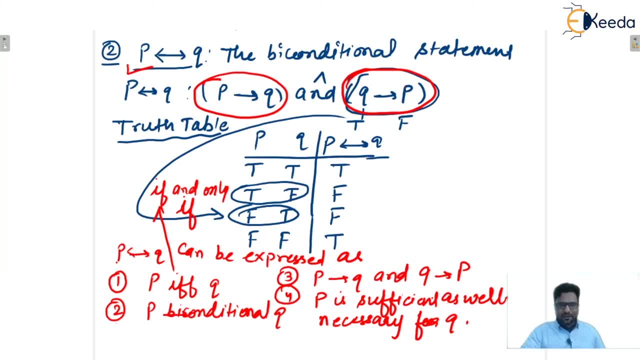 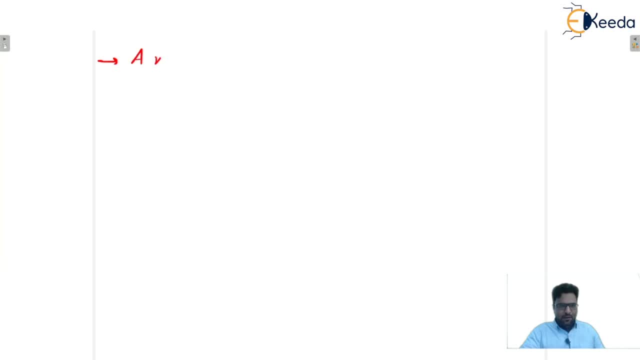 right, as well as right to left. Okay, So let us take one example on this. Yes, Let us consider one statement. Let's say a number. yes, we can say that being divisible by two, we can say: that is not only sufficient. 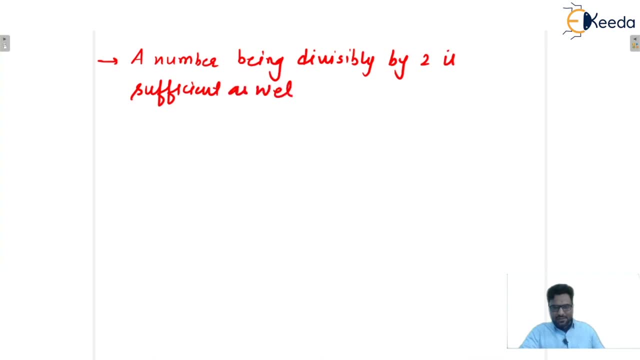 for Q, but it is also sufficient for P. So we can say that, being divisible by two, yes, we can say that, as well as necessary Yes or no For it to be even Yes or no. So we can say that this one is biconditional, Isn't it P? biconditional Q, where P is a number being. 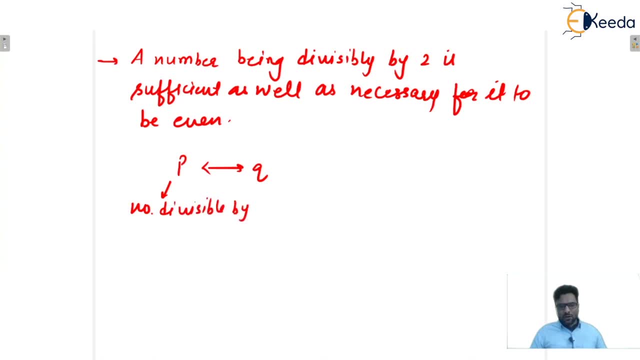 divisible by two, Yes or no, And Q is what. We can say: that it is even, Yes or no. So we can say that, left to right, if a number is divisible by two, then it is even. And we can say: 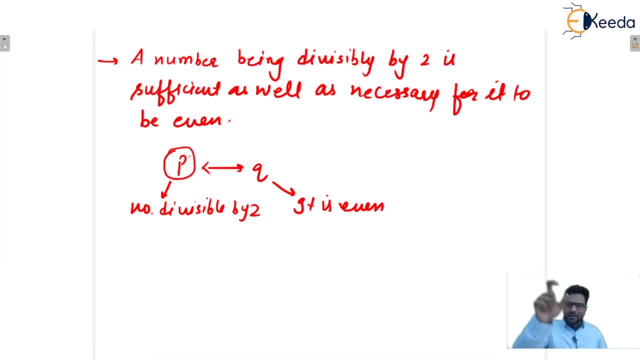 from right to left as well. if it is even, then it will be divisible by two. That is the meaning of biconditional. Here we can say that, yes, in the last example you seen, P implies Q. Yes, 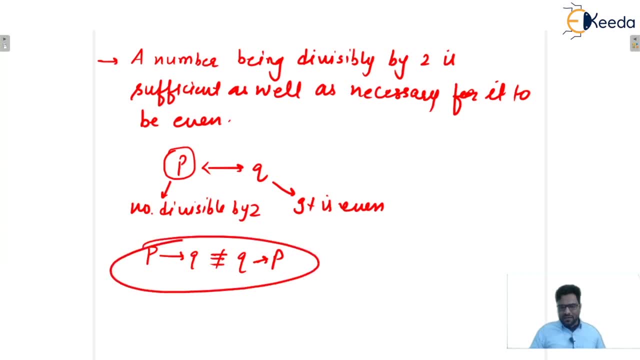 is not equivalent to Q implies P. Yes or no, We cannot say, because in the last example we seen, P implies Q doesn't mean Q implies P. I hope this one is clear to everyone. Okay, So let us take one.